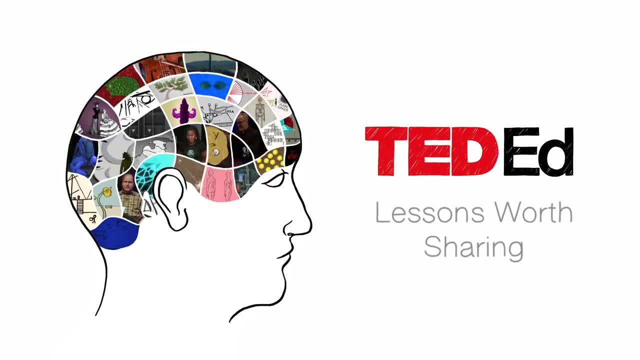 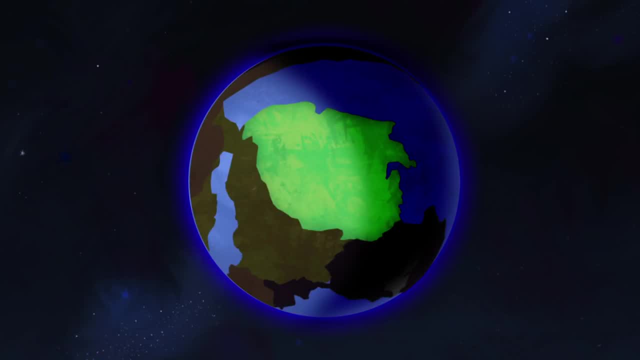 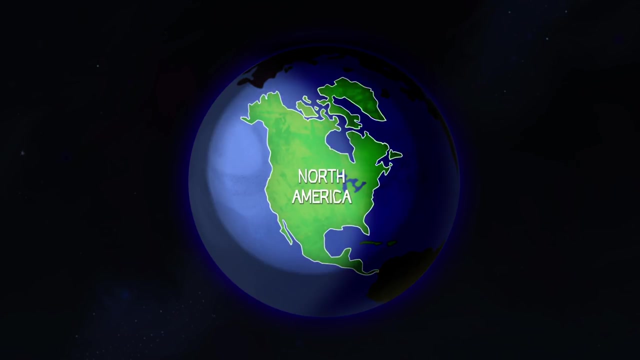 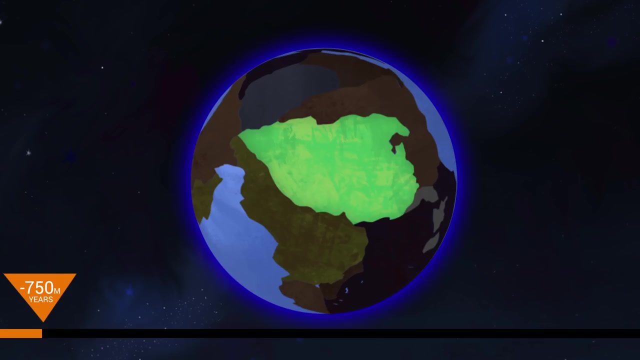 The geography of our planet is in flux. Each continent has ricocheted around the globe on one or more tectonic plates, changing quite dramatically with time. Today, we'll focus on North America and how its familiar landscape and features emerged over hundreds of millions of years. 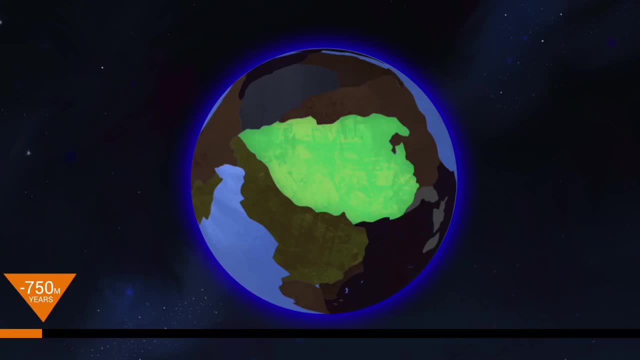 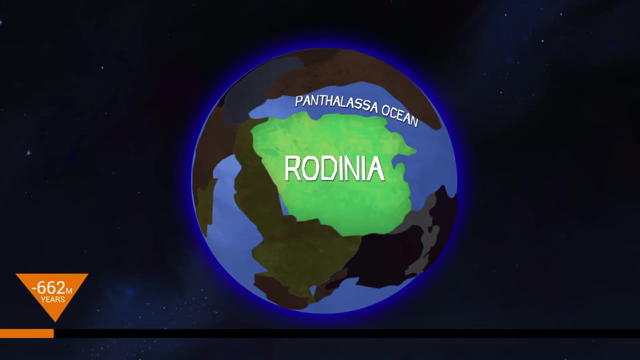 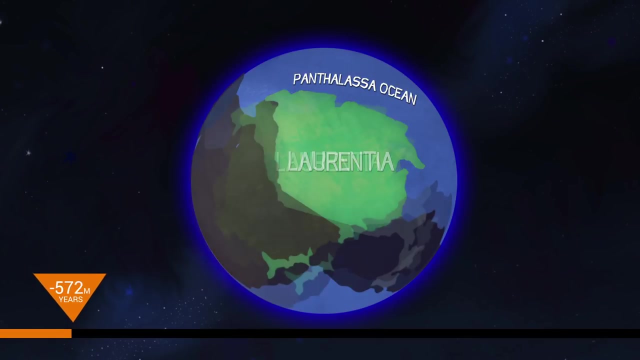 Our story begins about 750 million years ago. as the supercontinent Rodinia becomes unstable, It rifts along what's now the west coast of North America to create the Pantelassa Ocean. You're seeing an ancestral continent called Laurentia which grows over the next few hundred million years. 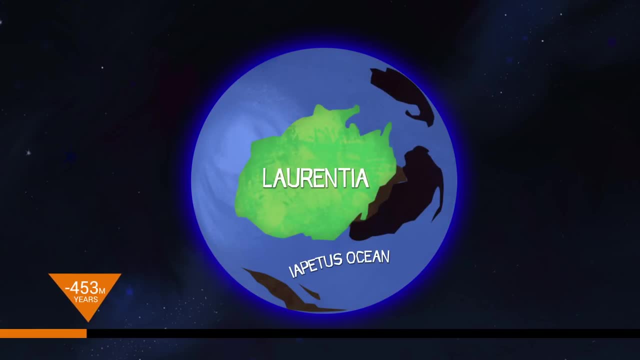 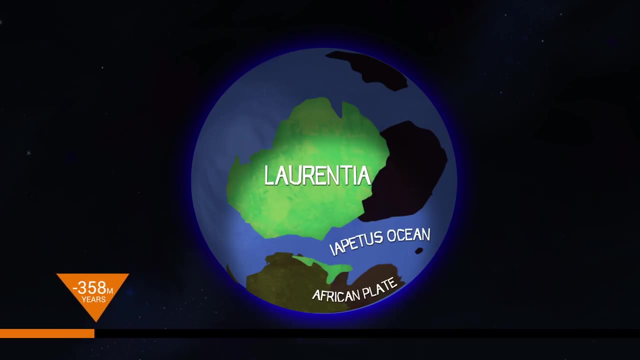 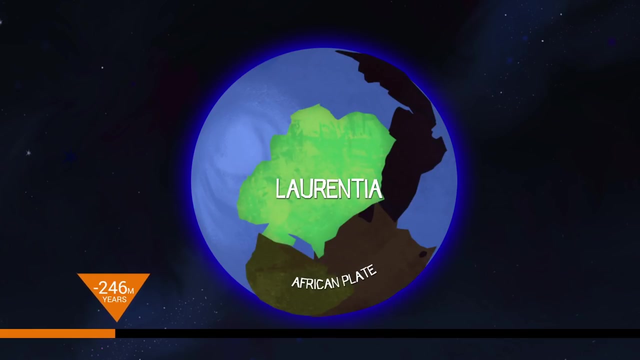 as island chains collide with it and add land mass. We're now at 400 million years ago. Off today's east coast, the massive African plate inches westward, closing the ancient Iapetus Ocean. It finally collides with Laurentia at 250 million years. 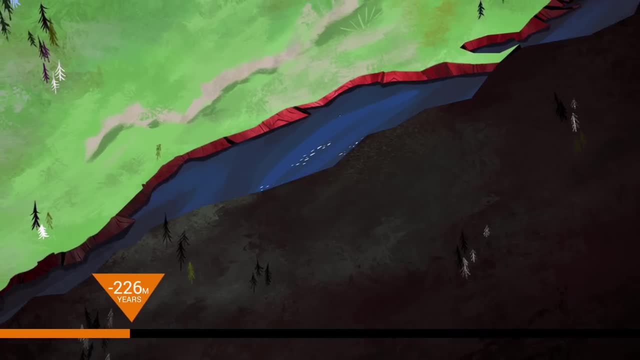 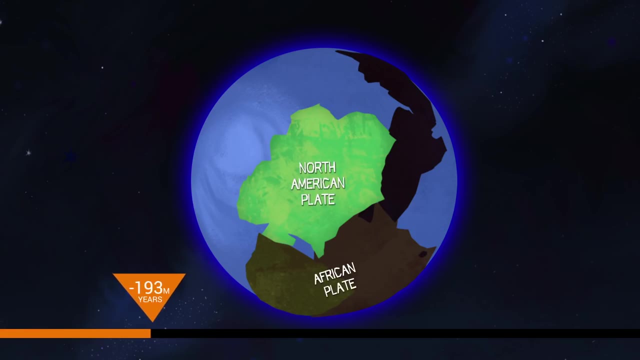 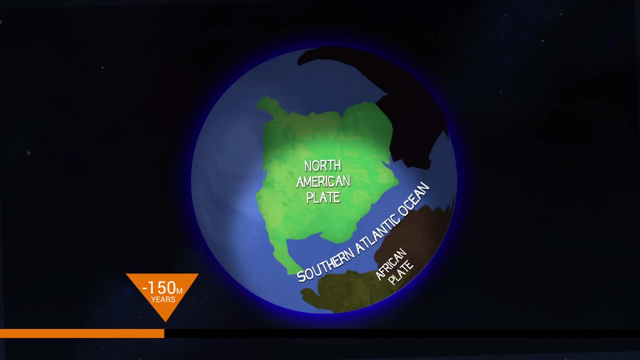 to form another supercontinent, Pangea. The immense pressure causes faulting and folding, stacking up rock to form the Appalachian Mountains. Let's fast forward a bit. About 100 million years later, Pangea breaks apart, opening the southern Atlantic Ocean. 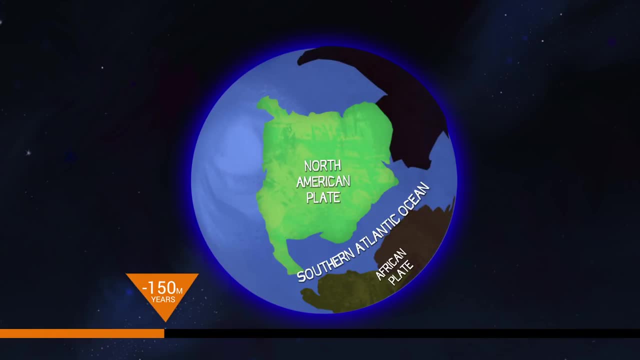 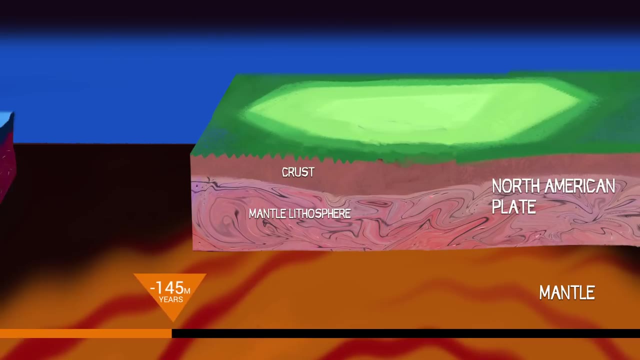 between the new North American plate and the African plate. We forge ahead, and now the eastward-moving Farallon plate converges with the present-day west coast. The Farallon plate's greater density makes it sink beneath North America. This is called subduction. 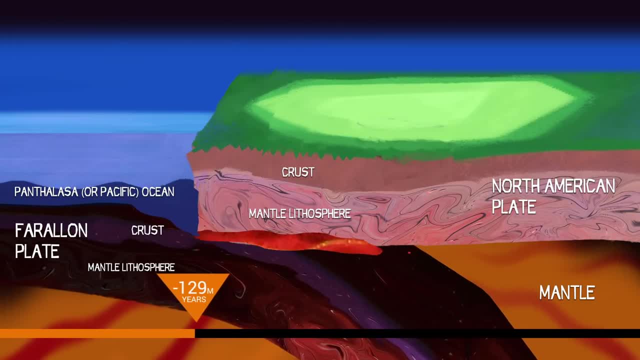 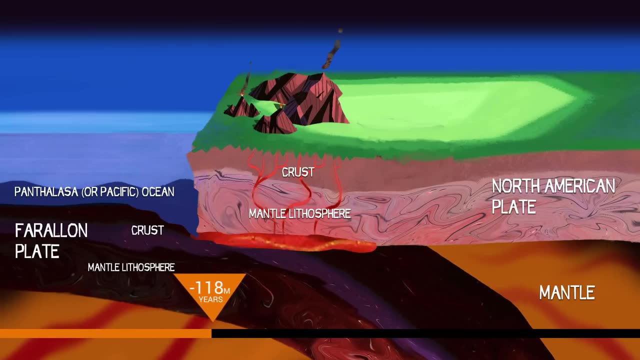 and it diffuses water into the magma-filled mantle. That lowers the magma's melting point and makes it rise into the overlying North American plate From a subterranean chamber. the magma travels upwards and erupts along a chain of volcanoes. 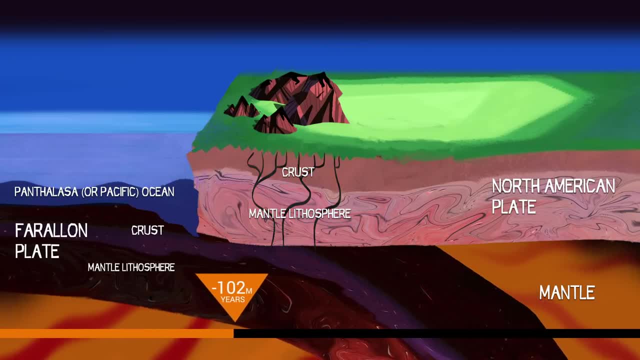 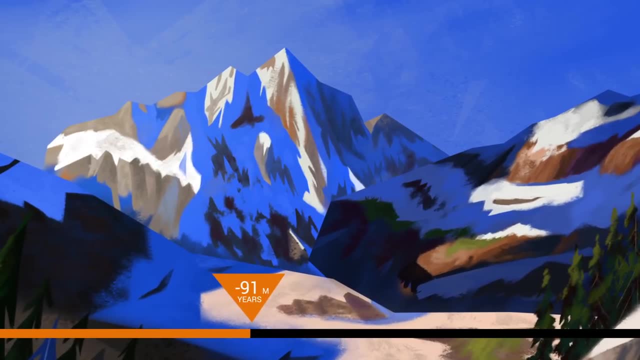 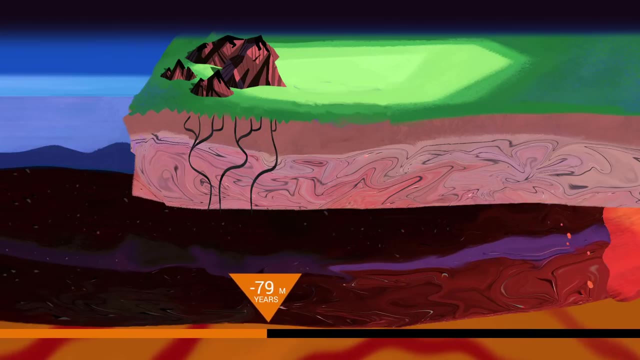 Magma, still deep underground, slowly cools, crystallizing to form solid rock, including the granite now found in Yosemite National Park and the Sierra Nevada Mountains. We'll come back to that later. Now it's 85 million years ago. The Farallon plate becomes less steep. 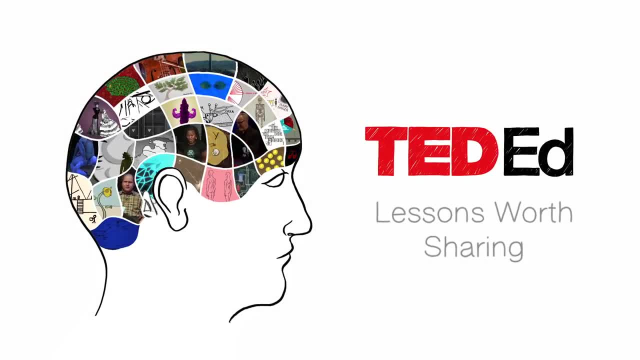 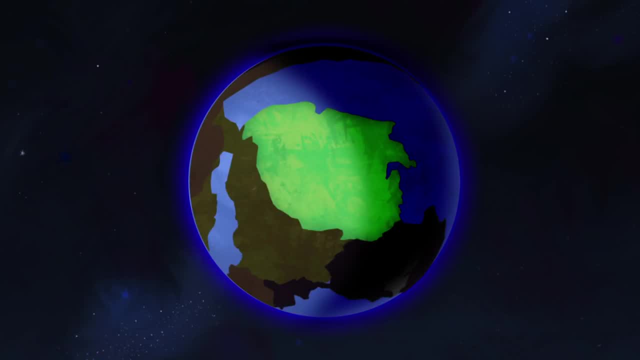 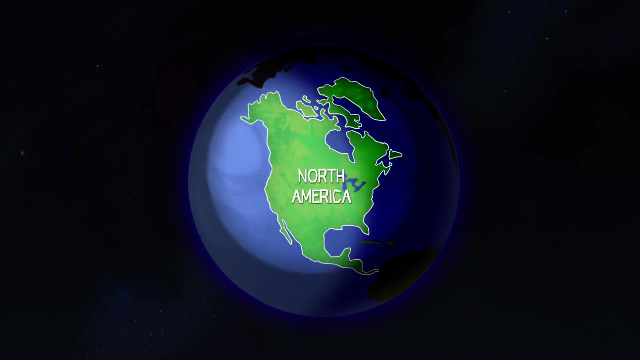 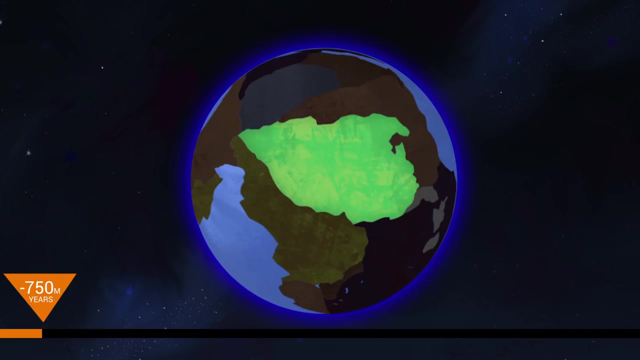 The geography of our planet is in flux. Each continent has ricocheted around the globe on one or more tectonic plates, changing quite dramatically with time. Today, we'll focus on North America and how its familiar landscape and features emerged over hundreds of millions of years. 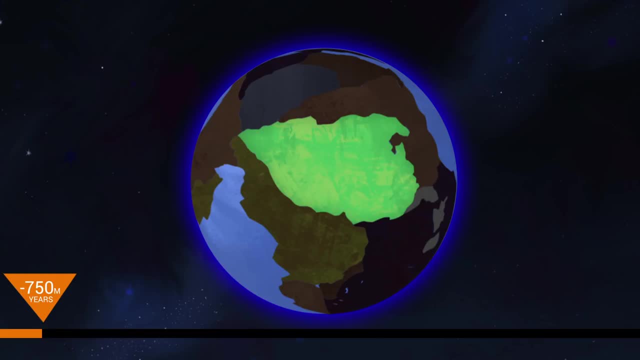 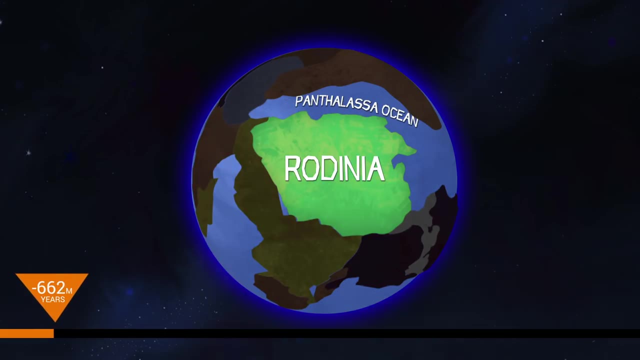 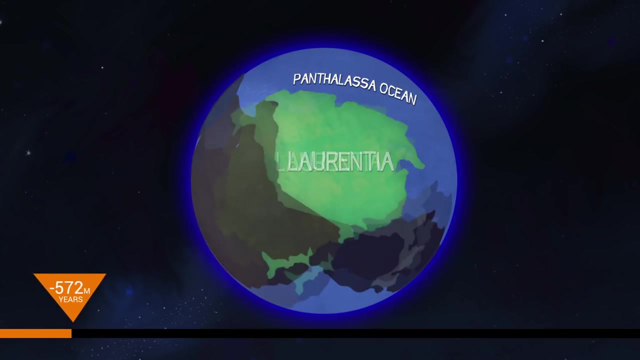 Our story begins about 750 million years ago. as the supercontinent Rodinia becomes unstable, It rifts along what's now the west coast of North America to create the Pantelassa Ocean. You're seeing an ancestral continent called Laurentia which grows over the next few hundred million years. 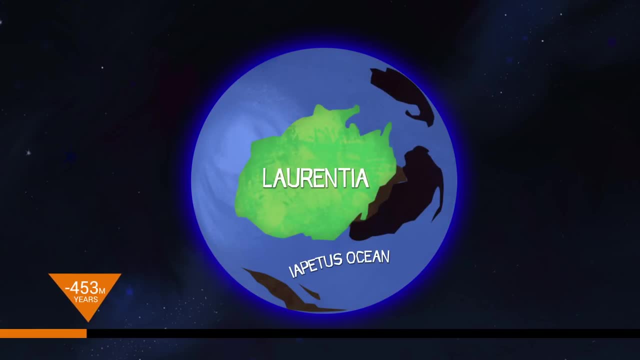 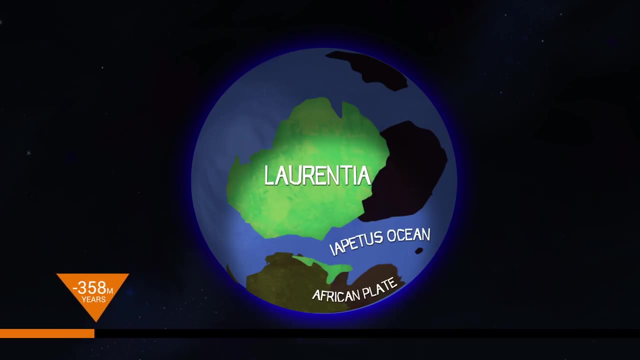 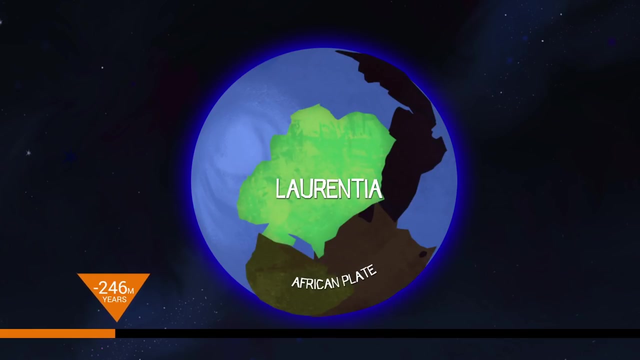 as island chains collide with it and add land mass. We're now at 400 million years ago. Off today's east coast, the massive African plate inches westward, closing the ancient Iapetus Ocean. It finally collides with Laurentia at 250 million years. 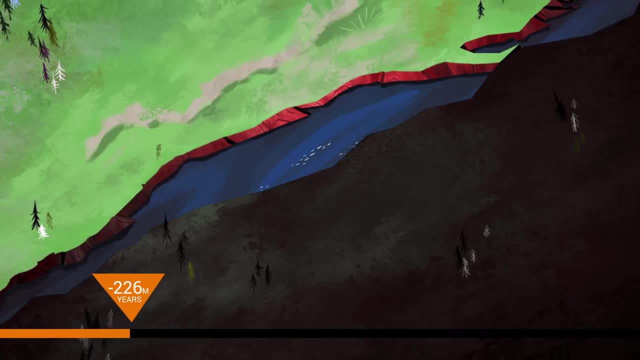 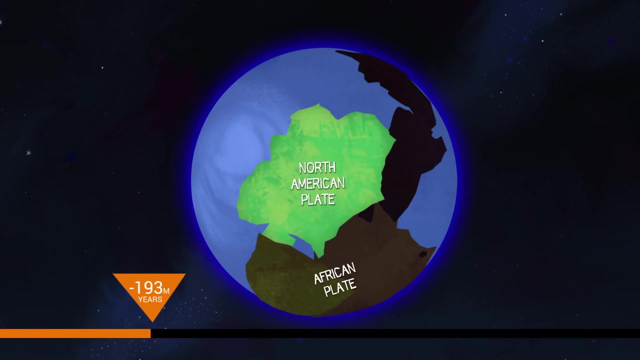 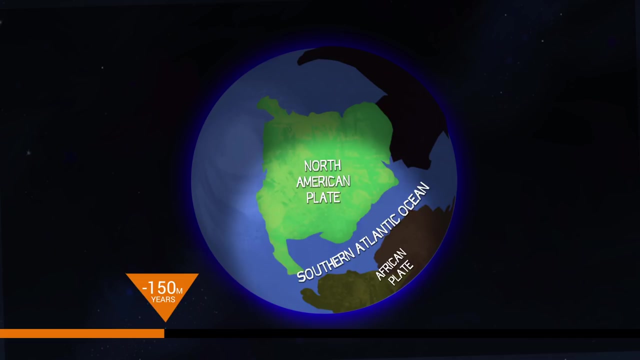 to form another supercontinent, Pangea. The immense pressure causes faulting and folding, stacking up rock to form the Appalachian Mountains. Let's fast forward a bit. About 100 million years later, Pangea breaks apart, opening the southern Atlantic Ocean. 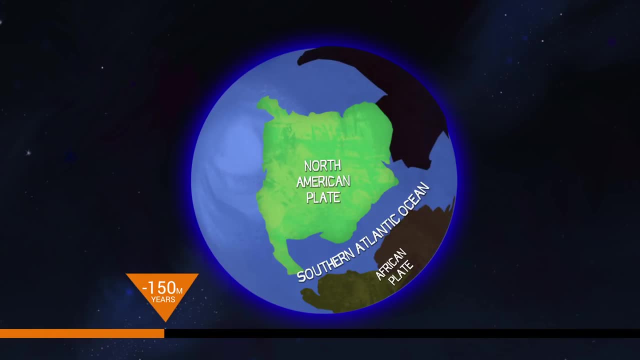 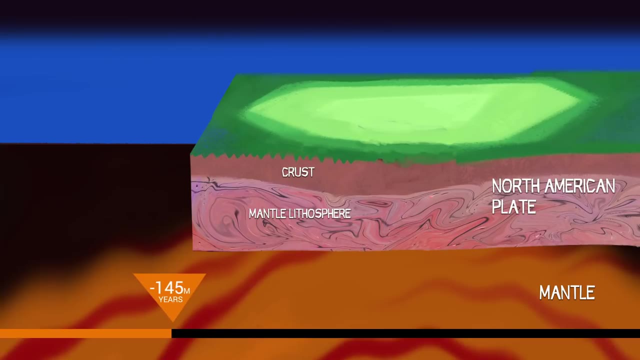 between the new North American plate and the African plate. We forge ahead, and now the eastward-moving Farallon plate converges with the present-day west coast. The Farallon plate's greater density makes it sink beneath North America. This is called subduction. 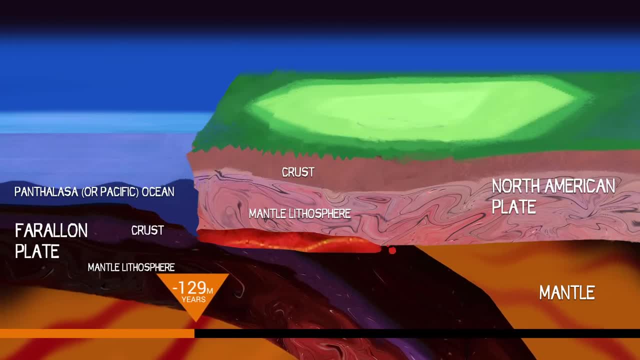 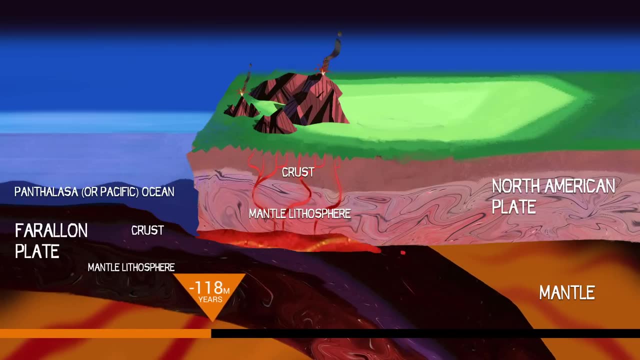 and it diffuses water into the magma-filled mantle. That lowers the magma's melting point and makes it rise into the overlying North American plate From a subterranean chain. the magma travels upwards and erupts along a chain of volcanoes. 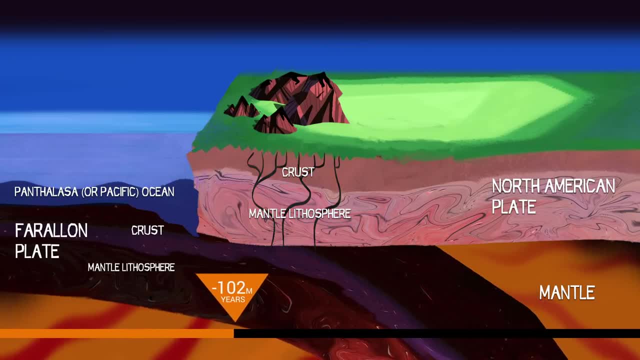 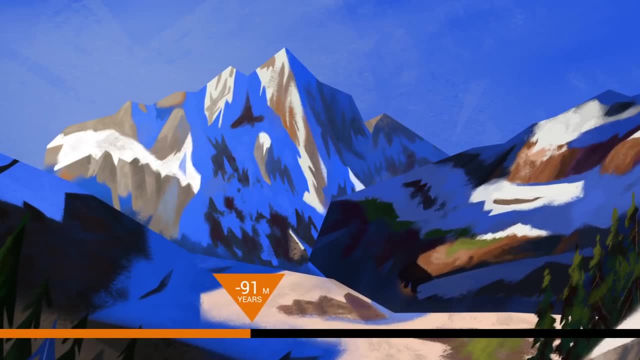 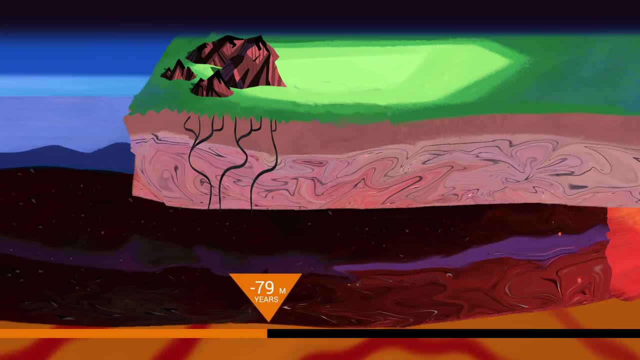 Magma, still deep underground, slowly cools, crystallizing to form solid rock, including the granite now found in Yosemite National Park and the Sierra Nevada Mountains. We'll come back to that later. Now it's 85 million years ago. The Farallon plate becomes less steep. 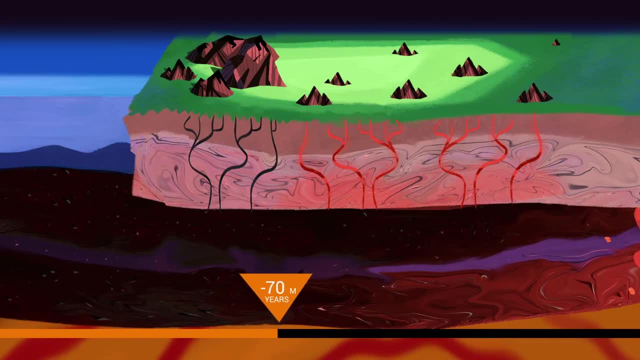 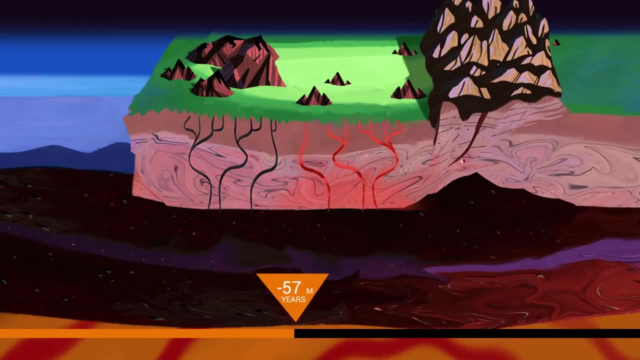 causing volcanism to stretch eastward and eventually cease. As the Farallon plate subsides, the Pangea plate becomes less steep and the Pangea subducts It compresses North America, thrusting up mountain ranges like the Rockies. 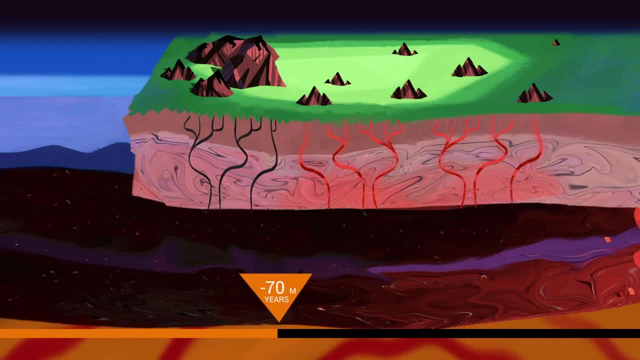 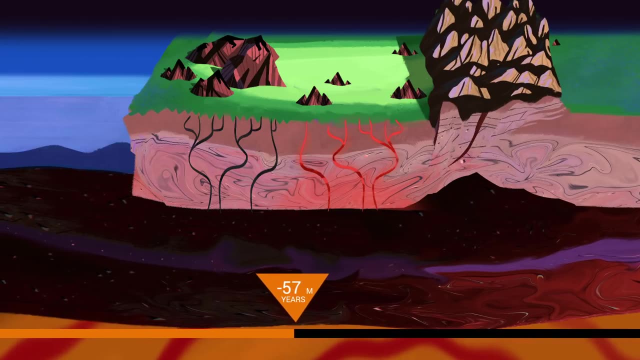 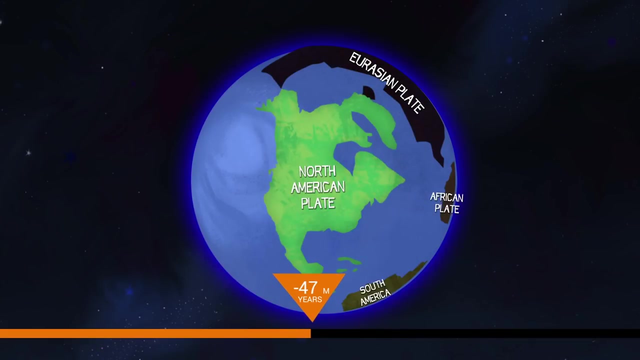 causing volcanism to stretch eastward and eventually cease. As the Farallon plate subdues, it compresses North America, thrusting up mountain ranges like the Rockies which extend over 3,000 miles. Soon after the Eurasian plate rifts from North America. 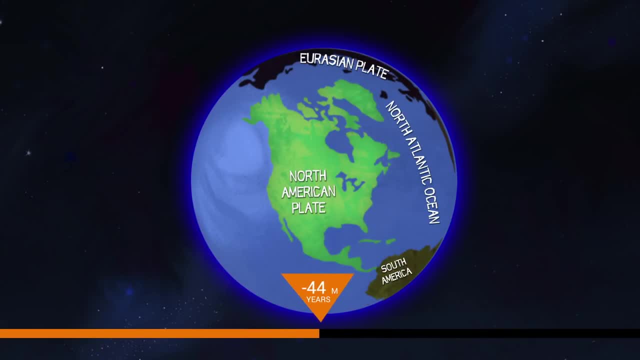 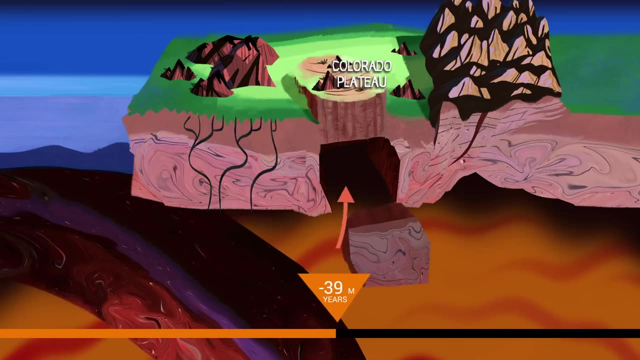 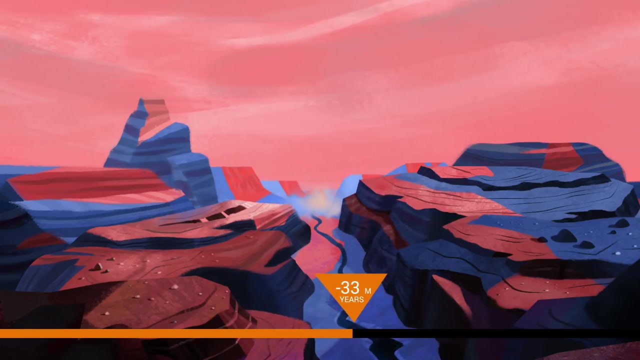 opening the North Atlantic Ocean, We'll fast-forward again. The Colorado Plateau now uplifts, likely due to a combination of upward mantle flow and a thickened North American plate. In future millennia, the Colorado River will eventually sculpt the plateau into the Eurasian Plateau. 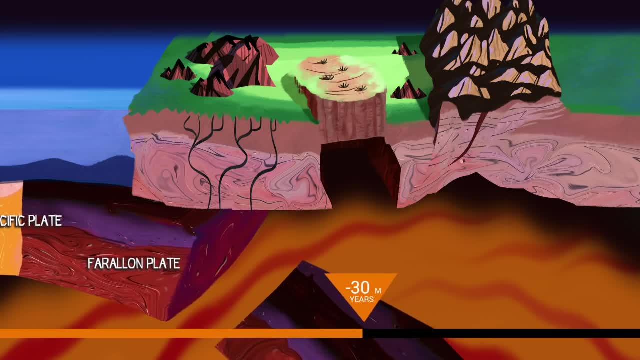 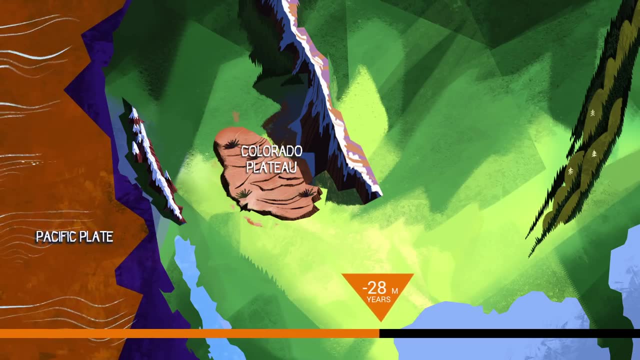 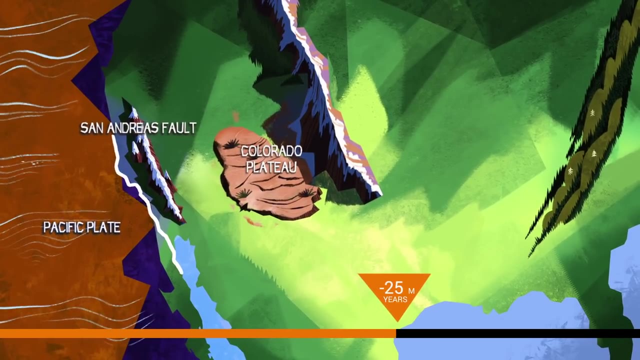 the epic Grand Canyon 30 million years ago. the majority of the Farallon Plate sinks into the mantle, leaving behind only small corners still subducting. The Pacific and North American plates converge and a new boundary called the San Andreas Fault forms. 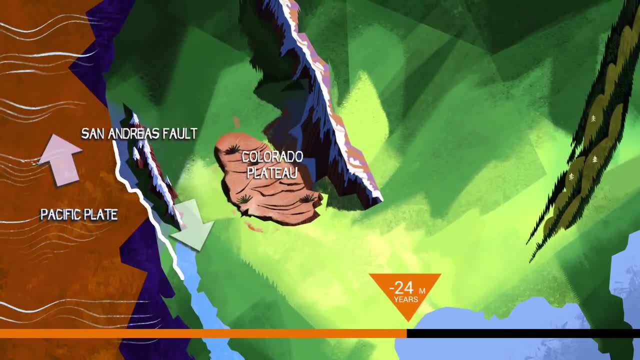 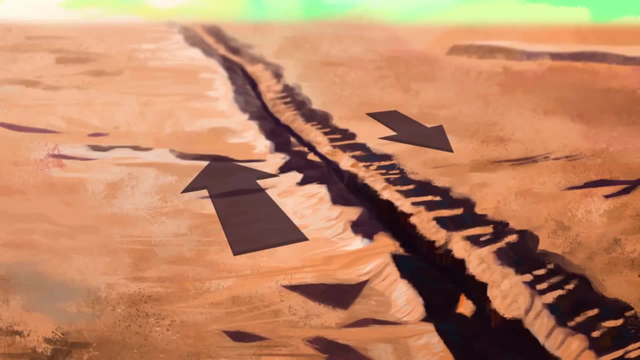 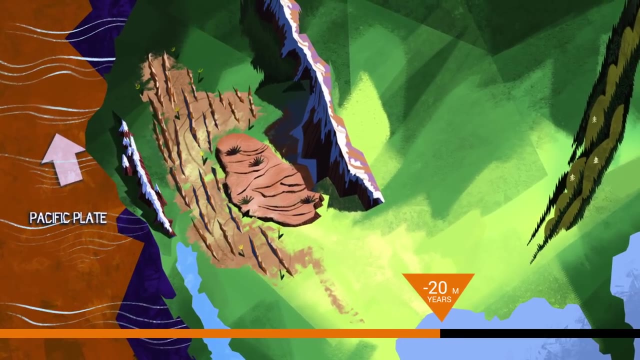 Here North America moves to the south, sliding against the Pacific Plate, which shifts to the north. This plate boundary still exists today and moves about 30 millimeters per year, capable of causing devastating earthquakes. The San Andreas also pulls apart western North America. 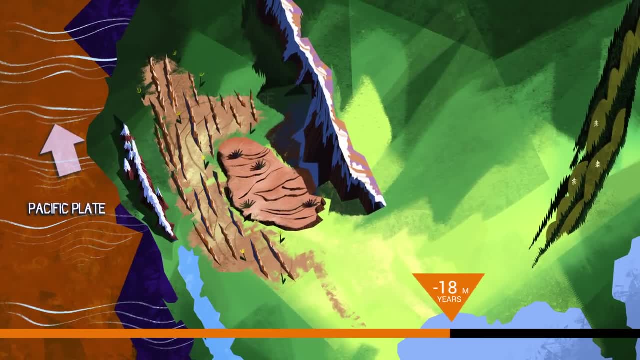 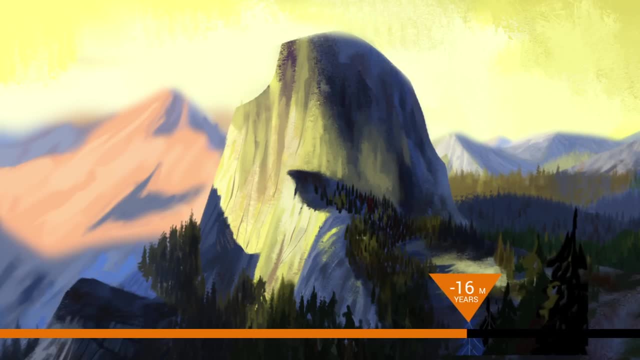 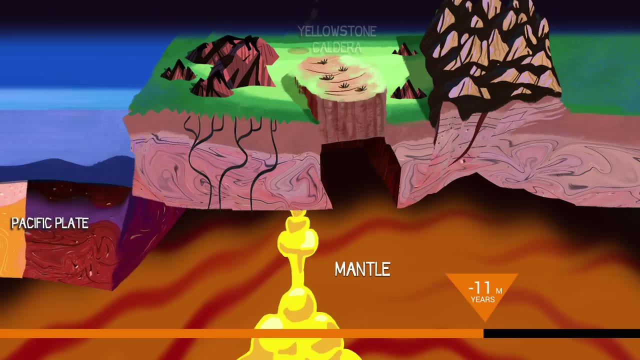 across a wide rift zone. This extensional region is called the Basin and Range Province and, through uplift and erosion, is responsible for exposing the once-deep granite of Yosemite and the Sierra Nevada. Another 15 million years off the clock and magma from the mantle burns a giant hole into western North America. 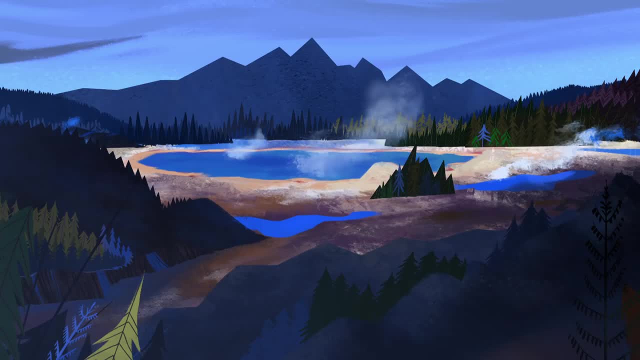 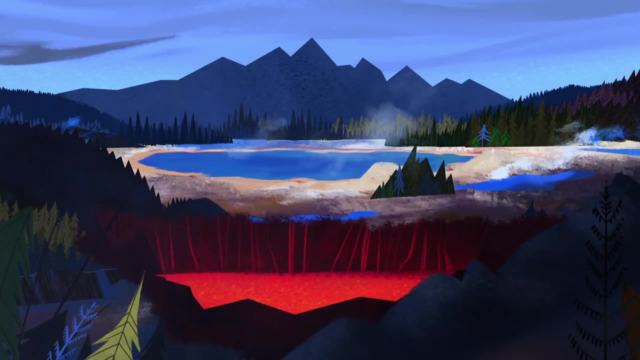 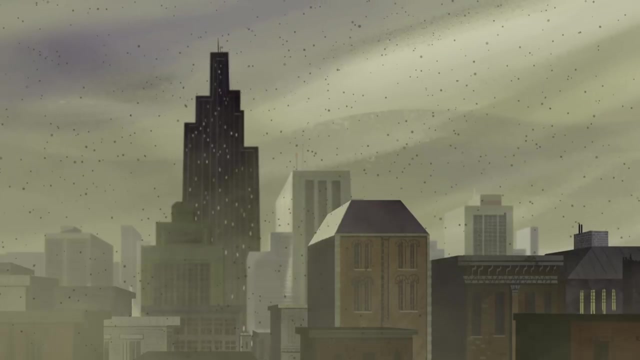 periodically erupting, erupting onto the surface. Today, this hotspot feeds an active supervolcano beneath Yellowstone National Park. It hasn't erupted in the last 174,000 years, but if it did, its sheer force could blanket most of the continent with ash. 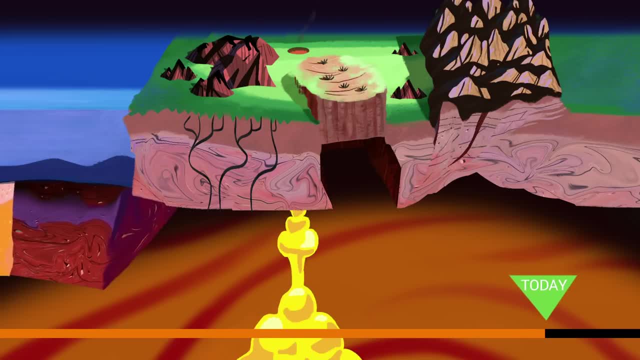 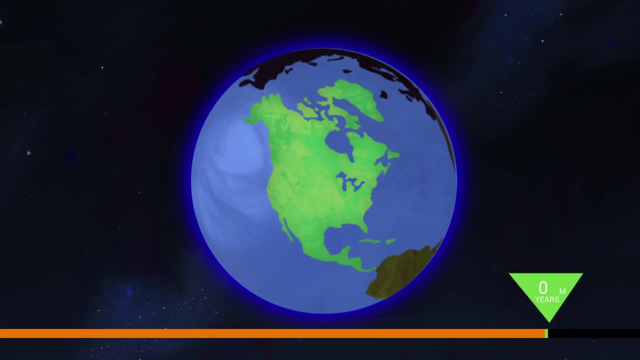 that would blacken the skies and threaten humanity. The Yellowstone supervolcano is just one reminder that the Earth continues to seethe below our feet. Its mobile plates put the planet into a state of constant flux. In another few hundred million years, who knows how the landscape of North America will have changed? 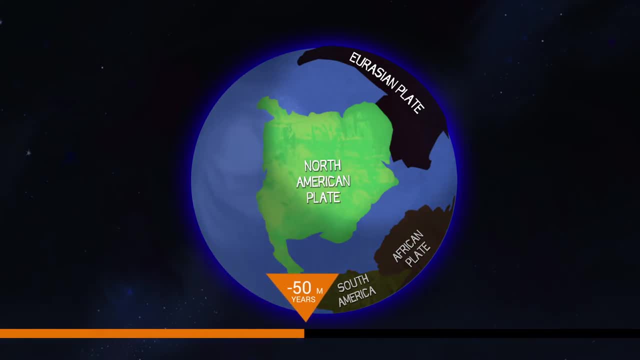 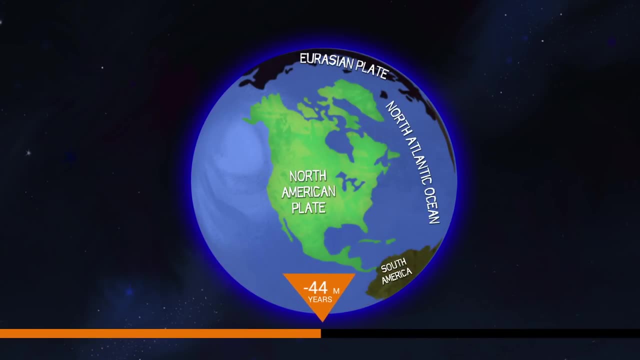 which extend over 3,000 miles. Soon after the Eurasian plate rifts from North America, opening the North Atlantic Ocean, We'll fast-forward again. The Colorado Plateau now uplifts, likely due to a combination of upward mantle flow. 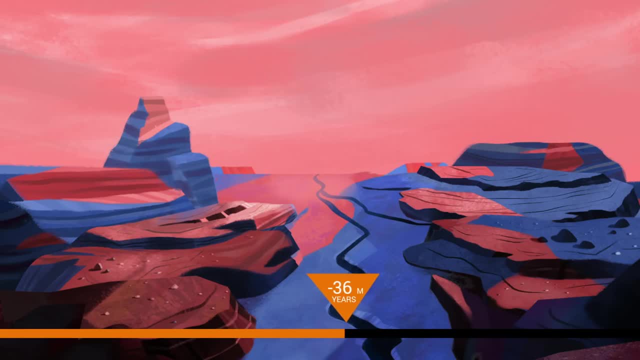 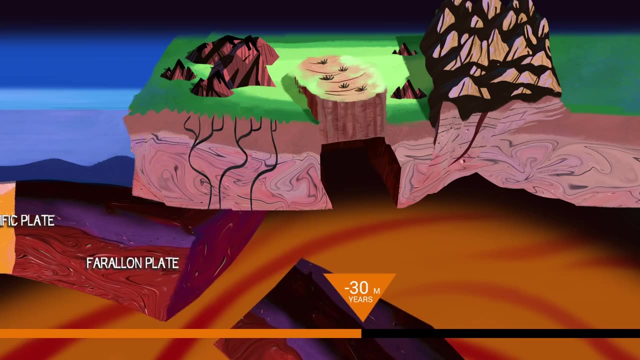 and a thickened North American plate. In future millennia, the Colorado River will eventually sculpt the plateau into the Eurasian Plateau. In future millennia, the Colorado River will eventually sculpt the Plateau into the epic Grand Canyon. Thirty million years ago. 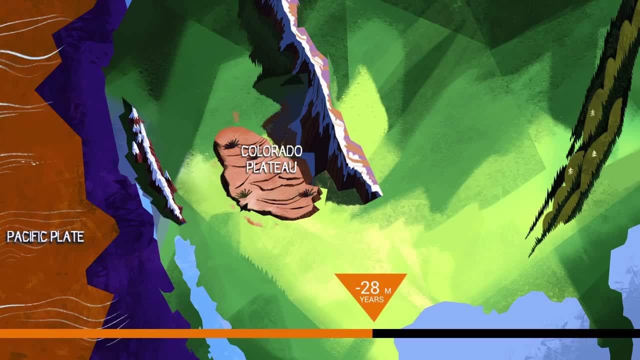 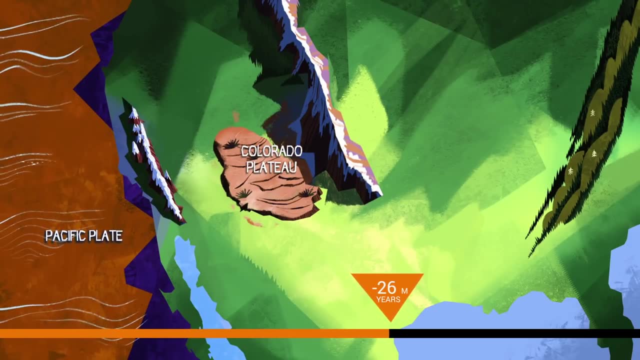 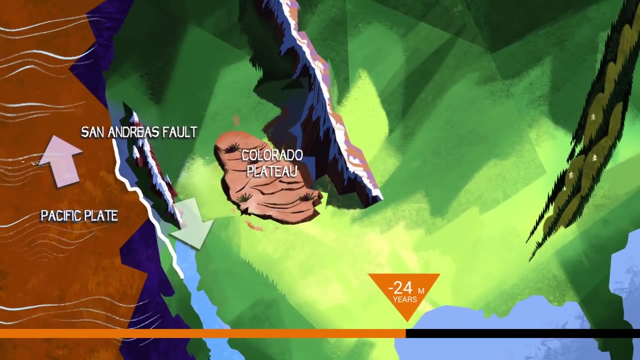 the majority of the Farallon Plate sinks into the mantle, leaving behind only small corners still subducting. The Pacific and North American plates converge and a new boundary called the San Andreas Fault forms. Here North America moves to the south, sliding against the Pacific Plate. 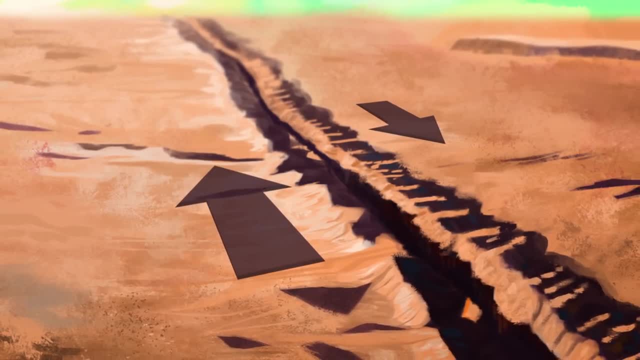 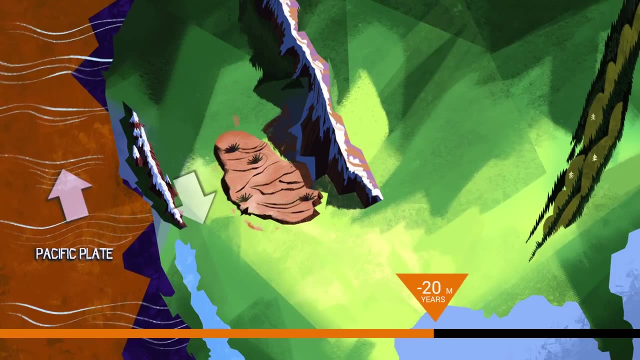 which shifts to the north. This plate boundary still exists today and moves about 30 million miles per hour and moves about 30 millimeters per year, capable of causing devastating earthquakes. The San Andreas also pulls apart western North America across a wide rift zone. 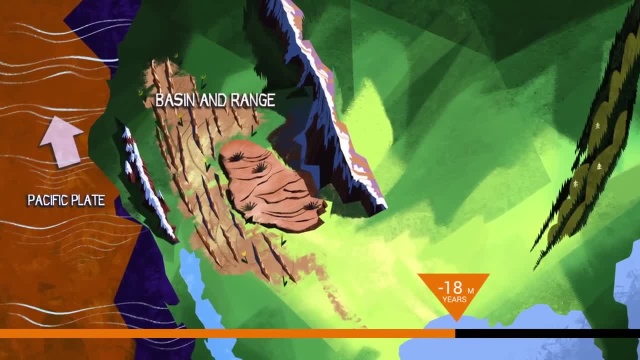 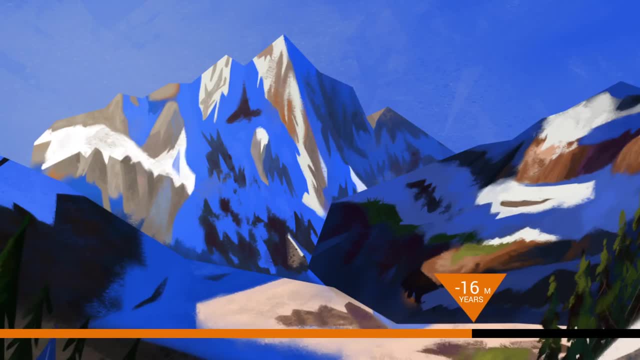 This extensional region is called the Basin and Range Province and, through uplift and erosion, is responsible for exposing the once-deep granite of Yosemite and the Sierra Nevada. Another 15 million years off the clock and magma from the mantle burns a giant hole into western North America. Another 15 million years off the clock and magma from the mantle burns a giant hole into western North America. Another 15 million years off the clock and magma from the mantle burns a giant hole into western North America. and magma from the mantle burns a giant hole into western North America. 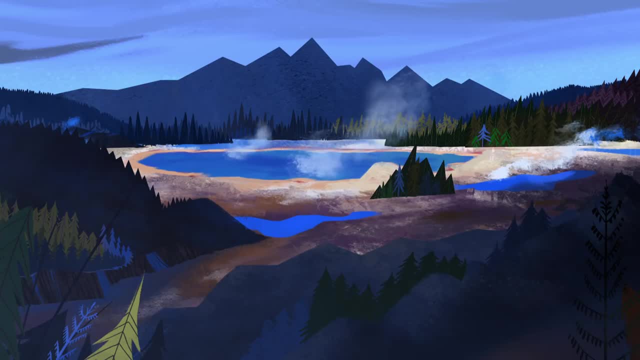 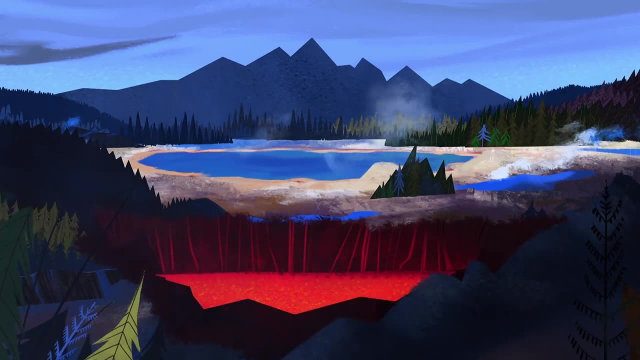 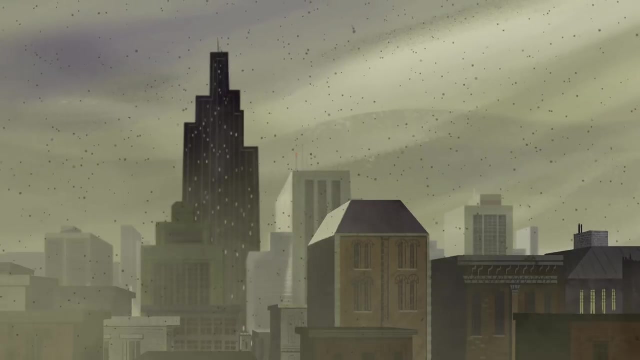 Periodically erupting onto the surface. Today, this hotspot feeds an active supervolcano beneath Yellowstone National Park. It hasn't erupted in the last 174,000 years, but if it did, its sheer force could blanket most of the continent with ash. 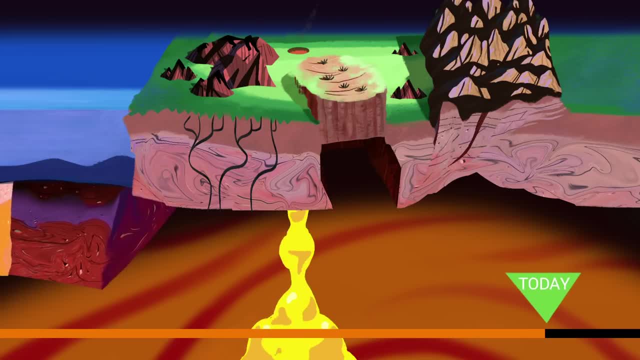 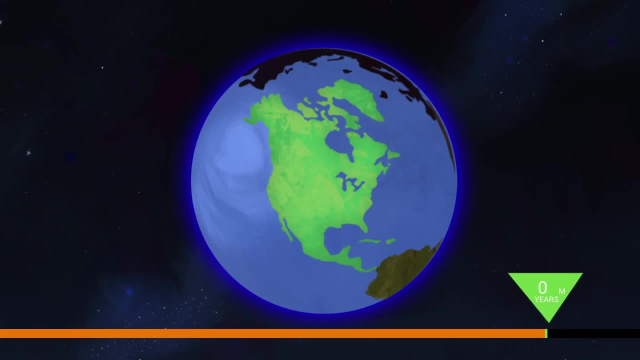 that would blacken the skies and threaten humanity. The Yellowstone supervolcano is just one reminder that the Earth continues to seethe below our feet. Its mobile plates put the planet in a state of constant flux. In another few hundred million years, who knows how the landscape of North America will have changed?